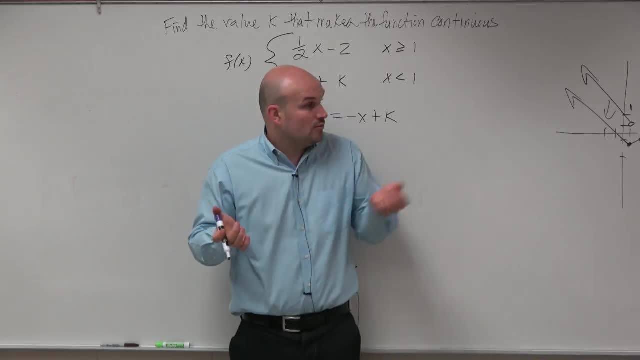 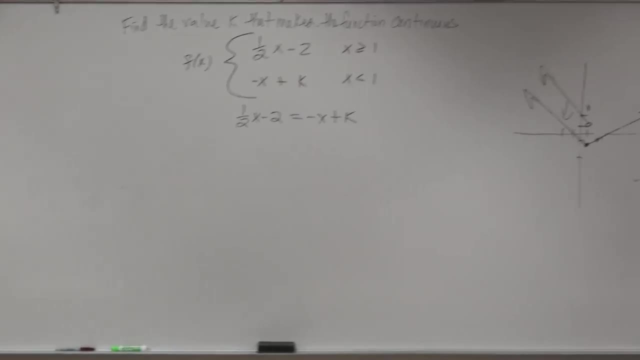 Set them equal to it. They have to be equal to each other If it's going to be continuous. whatever, the left side graph and the right side graph have to be the same, correct, They have to be equal to each other Now. 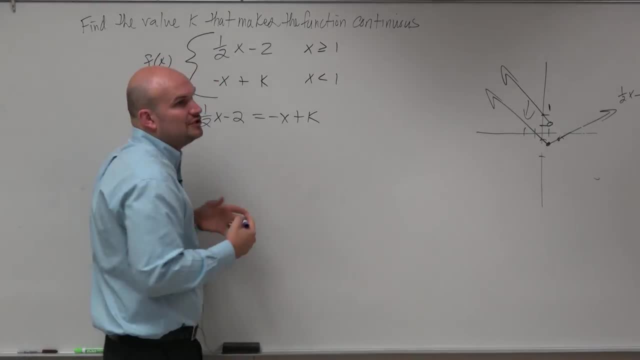 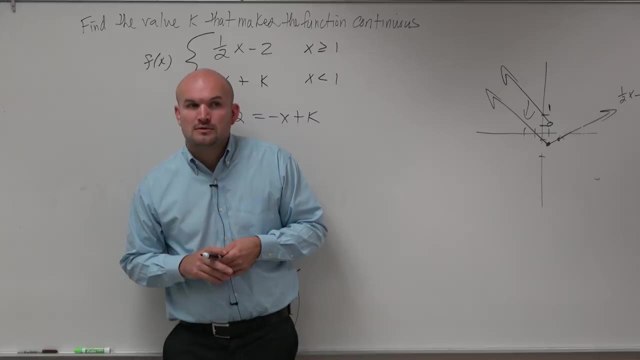 Now that they have to be equal to each other. what value of x are we trying to make them equal to each other? At what value of x are we trying to make them equal to each other? Where are they trying to meet at? At well, we don't assume you don't know the y value. 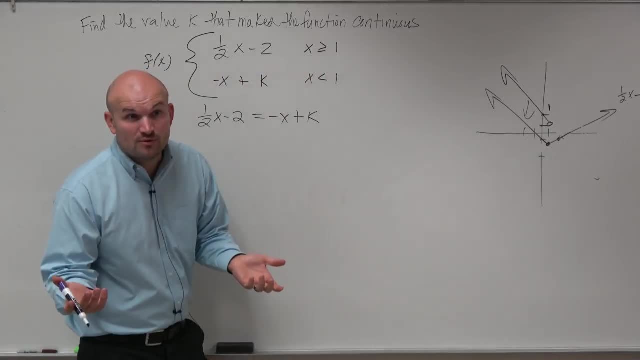 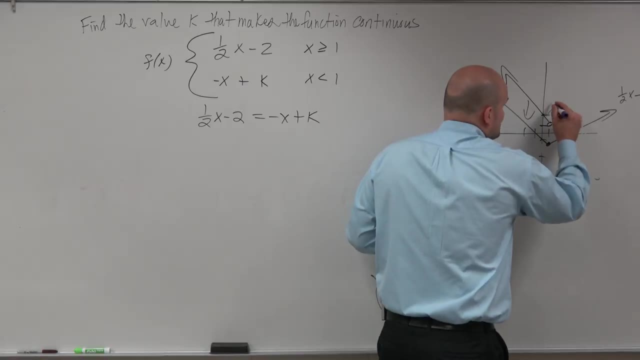 What x value are we trying to make Now again, negative 2 is the y value, but there's nothing for y. At what x value are they trying to meet at? Yes, Gabriel, 1.. 1. At x equals 1 is where they're going to connect right. 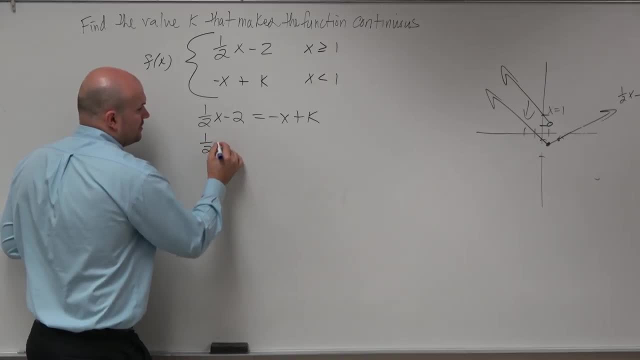 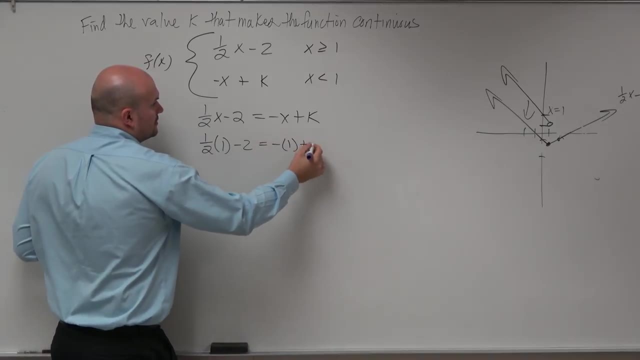 So. So what we're going to want to do is plug in 1 in for x, And again the reason why 2, I won't say it just because you know like you're saying that, because you can see it. 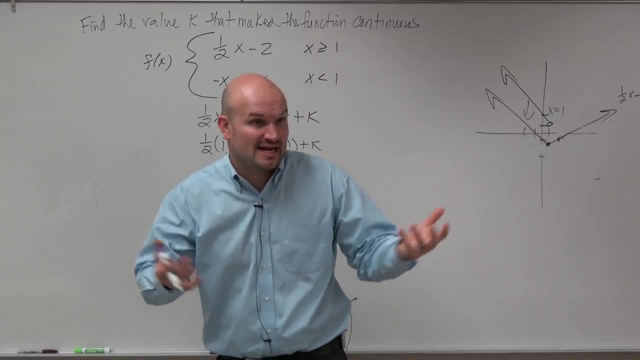 But imagine if I gave you something really crazy. you wouldn't know whether it would possibly connect. The only thing you would know is 1. And 1 is always going to be obvious because that's part of the piecewise function, right? 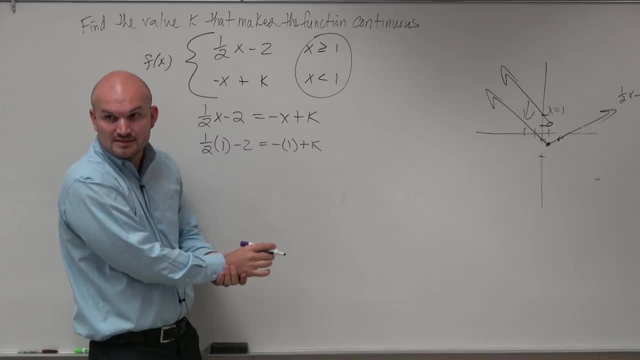 If I change this to 3, then you'd put 3 in for the x's. Does that make sense? Right, Yeah, So now all we've got to do is solve for k, And I chose a problem that we have. 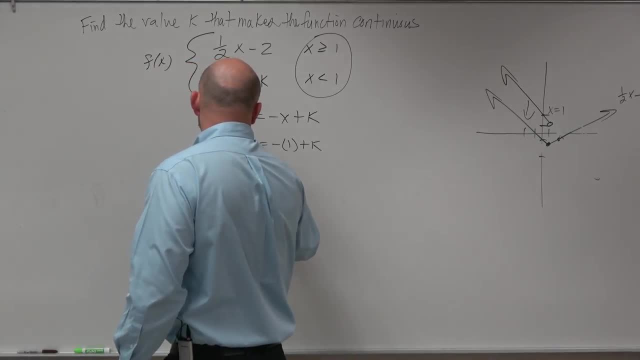 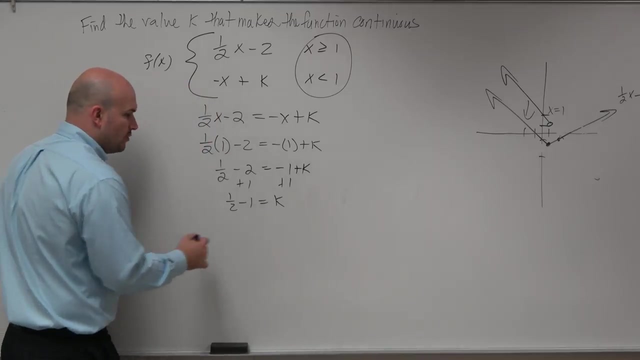 to deal with some fractions, because I like you guys that much. So 1 half minus 2 equals negative, 1 plus k. So I add 1, add 1 to both sides. 1 half minus 1 equals k. Well, 1 half minus 1 is going to be negative. 1 half equals k. 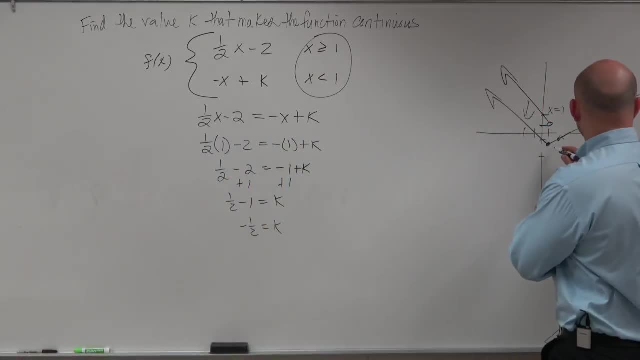 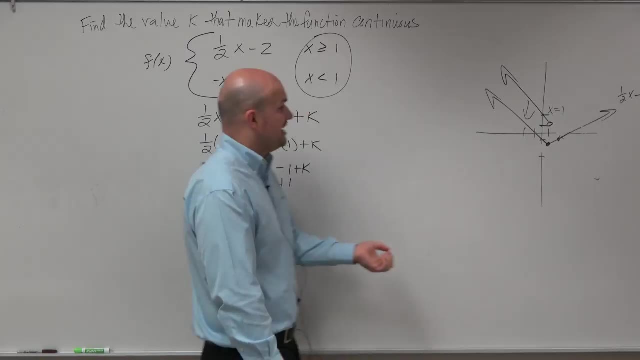 So what that means is if this graph- and actually, oh, we're going to use the y-intercept here, Oh, actually, yeah, you don't even know that's the y, That was the y-intercept- was that negative 2.. 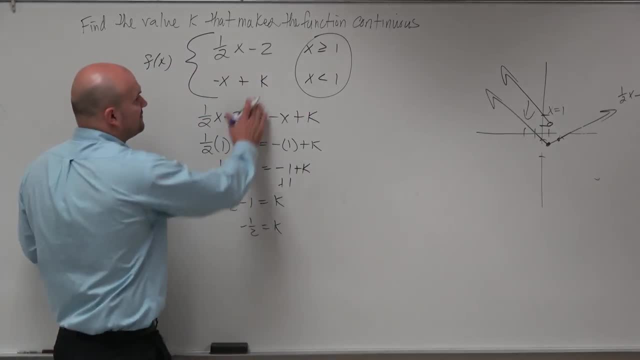 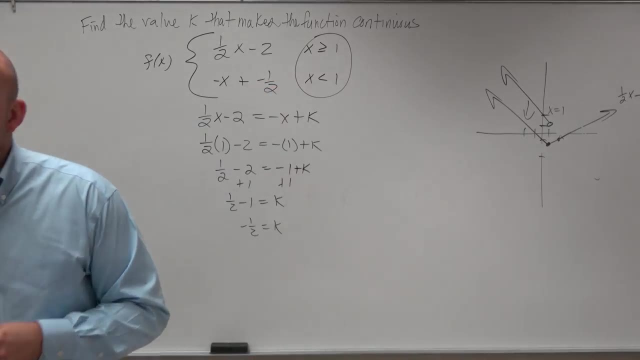 You actually don't know where that y-value is right there, But it ends up being. if you had this y-intercept at negative 1 half, if you guys were to graph these two now, they would be continuous function, And that's what the k is doing. OK, So before we go to lunch,